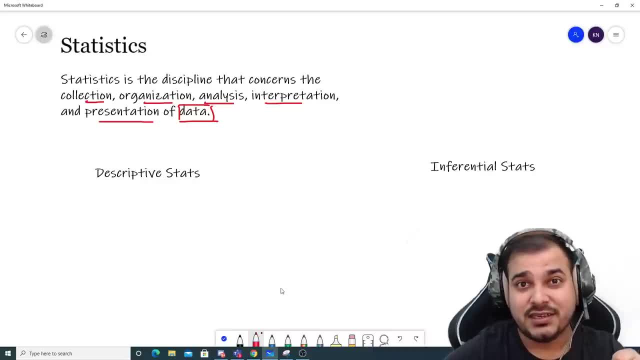 you understand what all things comes in this particular statistical terms. we are going to understand some of the mathematical terms too, you know. so, to understand what are the different types of statistics, we have two different types. One is descriptive stats and the other one is something called as inferential stats. Now, with respect to descriptive stats, 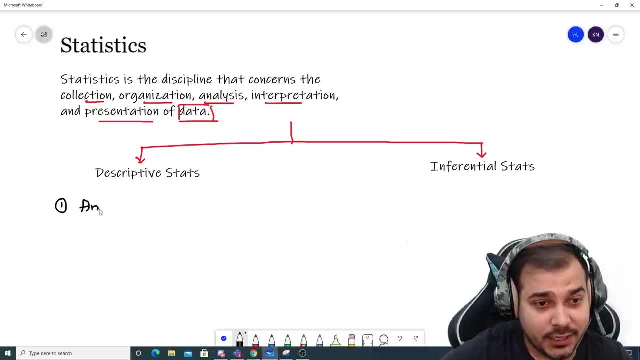 it actually involves, you know, analyzing the data. analyzing data, i can also say summarizing data- right, summarizing data, okay. or it can also be organizing data- right. we can do a lot of stuff with respect to descriptive strategy. still, i'll make you understand the. what is the exact difference between descriptive and inferential? 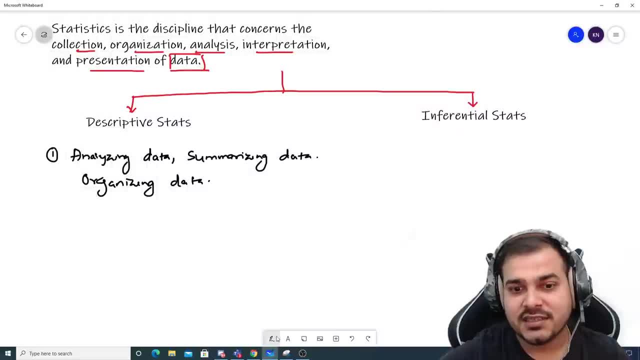 but please just understand that in descriptive statistic, it focuses more on summarizing the data, analyzing the data, organizing the data in the form of numbers and graphs, in the form of, in the form of: i'll write it in red color: number and graphs. this is very, very much important. 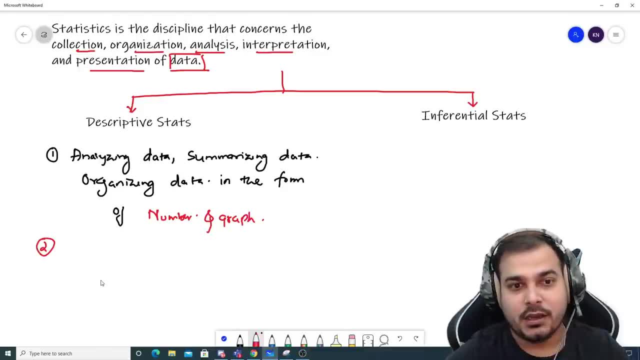 now, when i, when i say with respect to number, if i'm trying to organize this particular data, or do the analysis of this particular data in numbers and graph, by what? all ways we can come up with different, different graphs, right? so i'll just try to say that in the form of numbers and graphs. in the form of numbers and graphs. 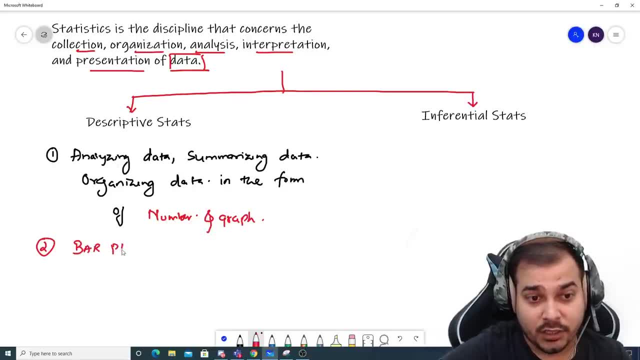 i'll try to show you. we have some of the example like bra plot, right, we have something like histograms. so these are our different, different types of plotting libraries. you know which we basically use? we use something called as pie chart, right, we? we use bar plot, uh, histogram, pie chart. 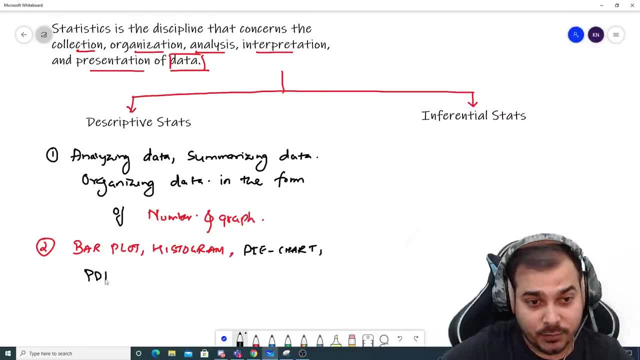 suppose i want to specifically use pdf, that is, probability density function, cdf, cumulative density function. so this kind of plotting graphs are basically used to analyze this kind of data, you know, to visualize this data right over here. visualization is also very, very much important because that visualization report from that particular 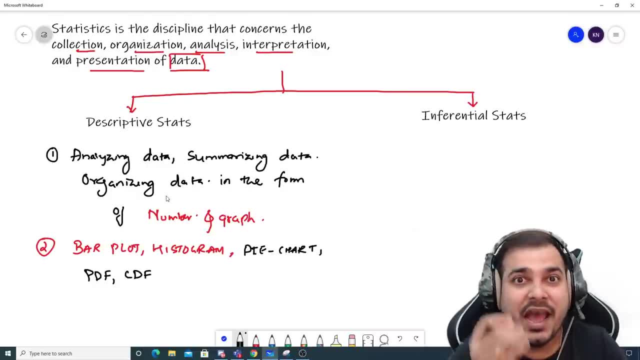 visualization stuff, we will be able to interpret some information and tell to our stakeholders, right? so all these things very important, important plot, you know we may talk about something like: uh suppose if i have a particular example, i may talk about normal distribution. based on the normal distribution or gaussian distribution, i may interpret some of the 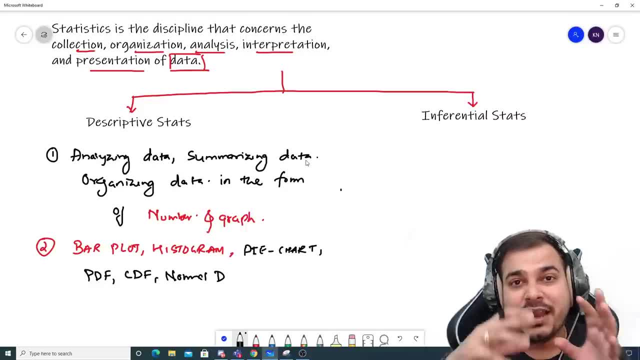 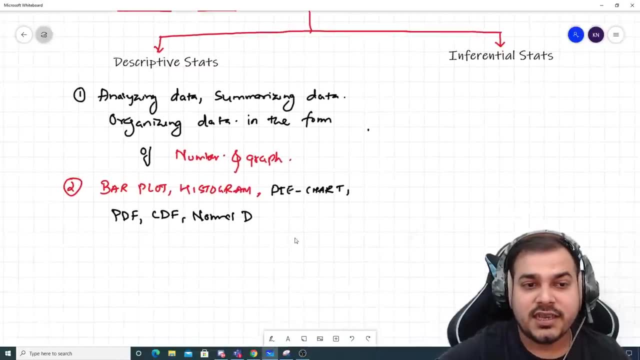 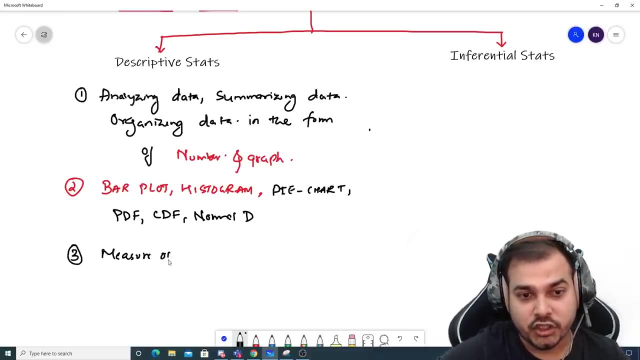 information, you know. so all those kind of interpretation, analysis, visualization can will be a part of this descriptive statistics. okay, uh, not only this, guys, if i include my third point. my third point is basically with respect to measure of central tendency. right, measure of central tendency. now, if you don't know about measure of central tendency, guys, i can talk about. 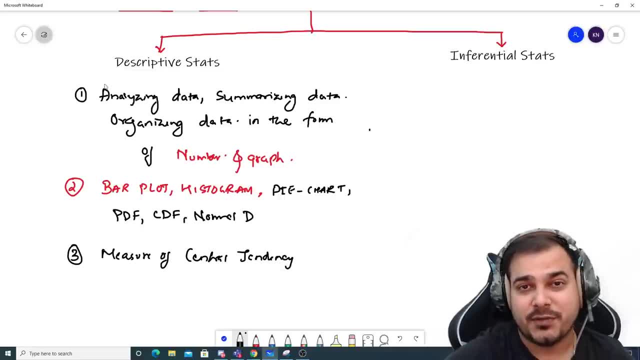 mean median mode. that also gets included in descriptive statistics. always remember, guys, whenever we talk about descriptive statistics, the first point is there is a measure of central tendency statistics. our data may be a population data also. it can be a sample data also. it is very, very much. 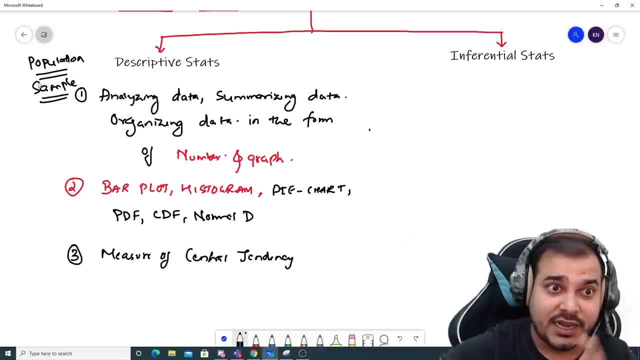 important to understand, guys. okay, it can be a population data, it can be a sample data. that basically means we can analyze the data sets with respect to both population and sample. we can apply this kind of plots to both this kind of data set. we may apply different type of measure of central. 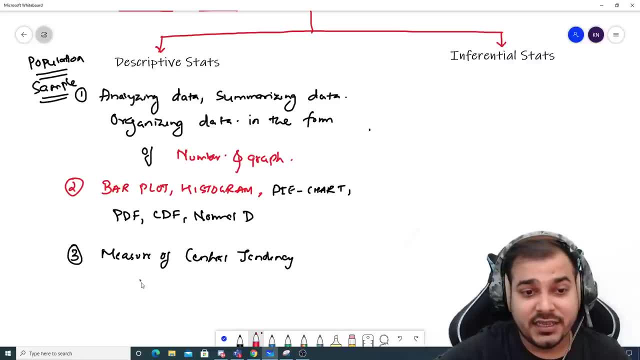 tendency like mean median mode. if i talk about central tendency, this is basically mean median mode, right? i hope everybody is familiar with this, because i have already made this kind of videos in my statistics playlist. right now, coming to the fourth point, you know there is also something. 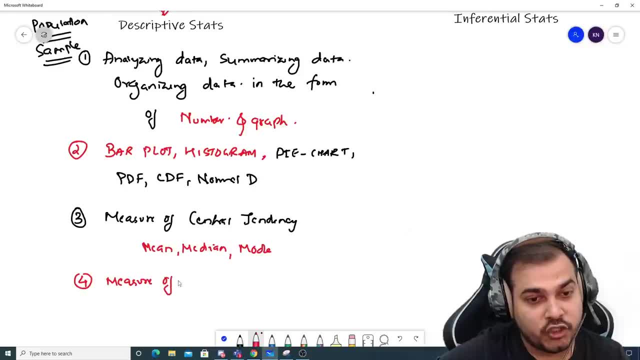 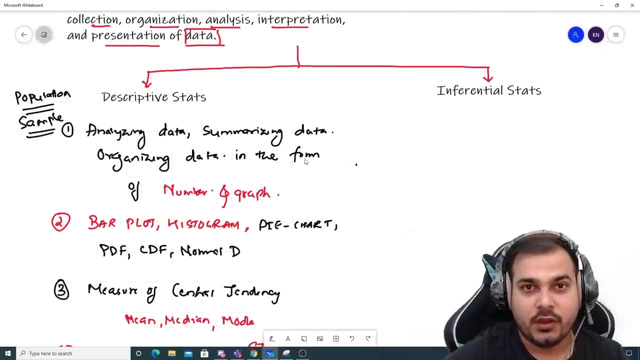 called as measure of variance. measure of variance right now, when i say measure of variance, obviously there is something called as standard deviation, there is something called as variance. all these things, you know, will definitely be a part of descriptive statistics. okay, it will definitely be a part of descriptive statistics. 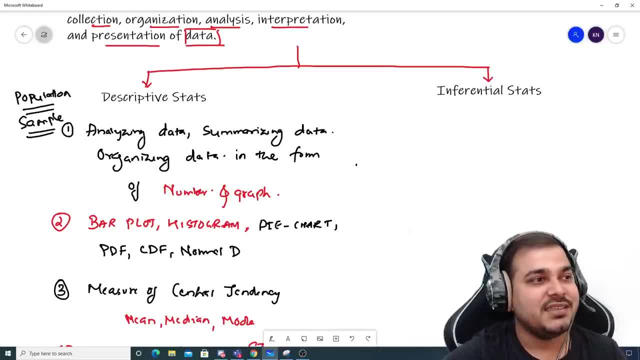 statistics. now, the main question that arises then: what is inferential statistics? right, inferential statistics? let me tell you guys, let's, let's take a very good example. suppose i have some kind of population data set, okay, suppose, let's, let's imagine that, uh, recently a election has. 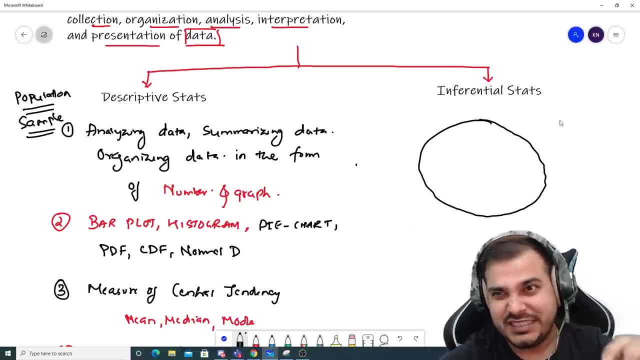 happened, uh, probably in west bengal, probably in one of the state in india, any place. okay, now, if we really need to find out what is the exit poll? exit poll is basically, uh, to find out the information, which party has the highest chances to win. you know now, suppose in. 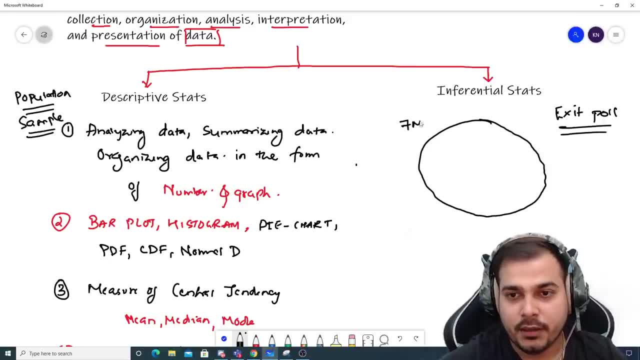 this particular state, there are somewhere around 7 million people. okay, we cannot go and ask each and every person that whom they have actually voted, you know. so what we do is that we try to just take a sample of this, probably, and we try to perform this exit poll, exit poll. what it does from different? 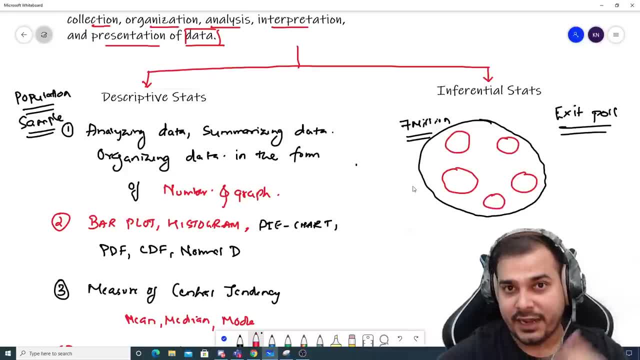 different location. they'll try to take a sample data and then tell they'll try to ask whom do you vote? okay, usually they'll try to take a sample data and then they'll try to ask whom do you vote? okay, but it's fantastic from this particular situation that they have seen. 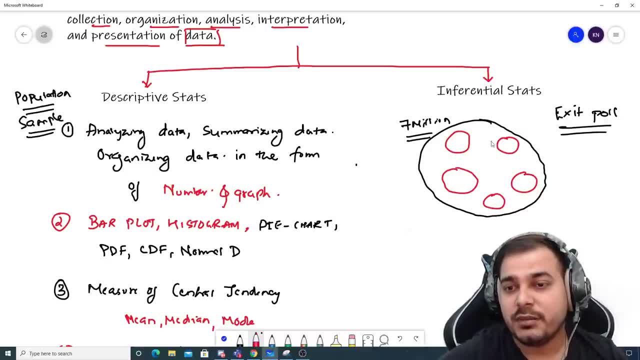 the news. people do do this, you know, when they want to take out this particular exit. pull now, suppose, from this particular population of, sorry, from this particular sample. remember, the seven million is basically my population, right, and this is basically my sample, which i have actually selected. now suppose from the sample says that, okay, from all the samples. says that: 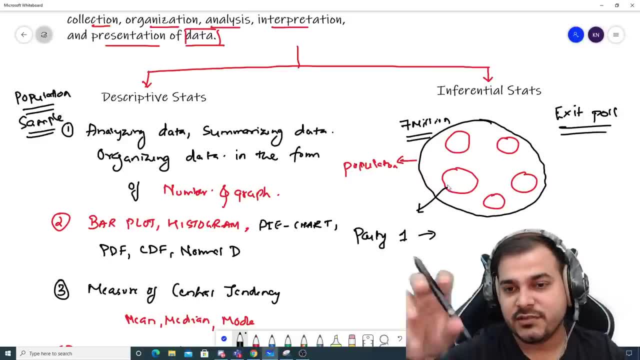 party one has will win probably this many seats. you know, we have just taken some sample of information from every part of this particular state, right? so now suppose if participating winning is so, they say that, okay, party one, the one, will win this many states, party two will win this minister. 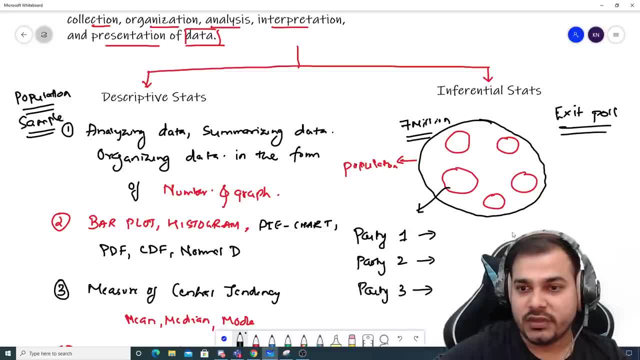 seats. you know party three will win this many seats, so then they will try to decide that. what is the percentage with respect to the exit poll, that people will be winning or the parties will be winning over there, right? so this particular information, what we are doing, from the entire. 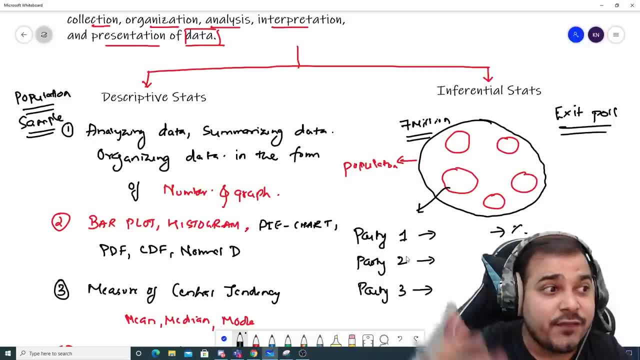 population. we are just taking a sample and we are inferencing some information. we are inferencing some information and we are coming to a conclusion saying that, okay, this party will win right. that is the important of influential statistics. so in inferential statistics, guys from the entire population you know, from the population you know. so i'll just remove this. 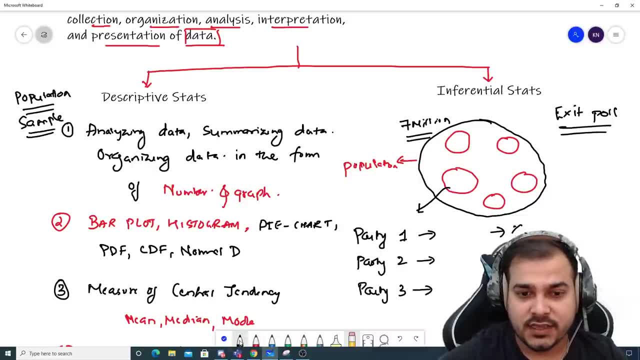 population. what we do in- uh, in this kind of things, is that we take a sample from a population and then we try to do some kind of test- okay, it can be any kind of test, okay. and then we come up with an inference and conclusions for that specific population, for that specific population. this 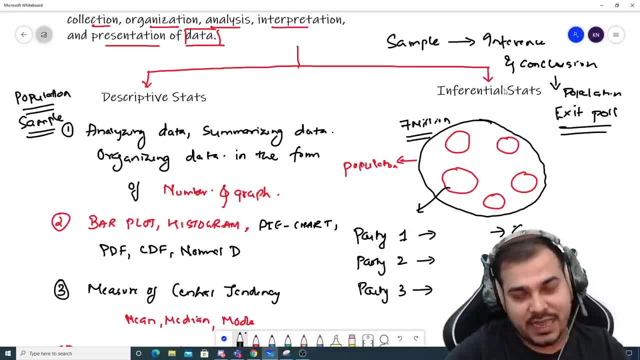 is very, very much important to understand right. we take the sample from that particular population, we use that particular sample data and we make an inference, we make a conclusion, we make a decision specific to that specific population. now, in this particular case, if I really want to find out the exit poll, I cannot go and ask each and every person whom. 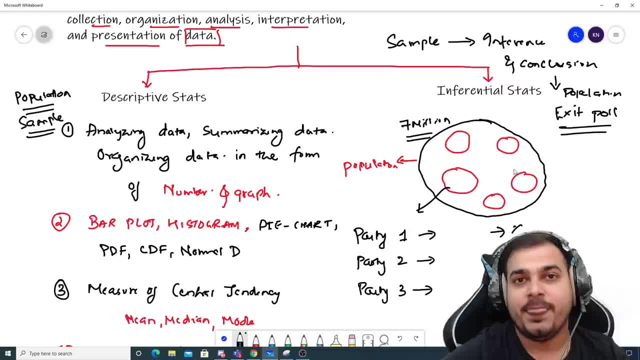 did you vote? so what I will do is that I will take a sample of this particular data and I will come to a conclusion and inference for the entire population. always remember an inferential statistic. there is also something called as confidential intervals, confidence intervals- right, so this is also very, very much important. that is called as confidence. 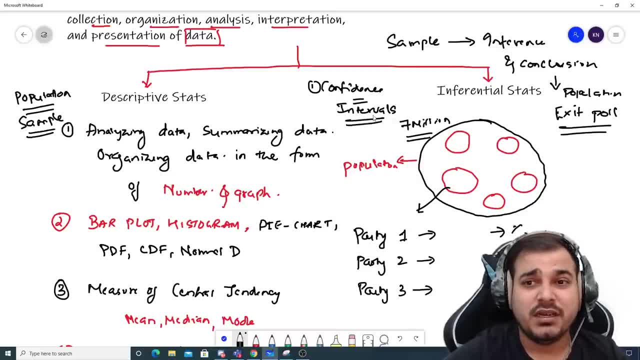 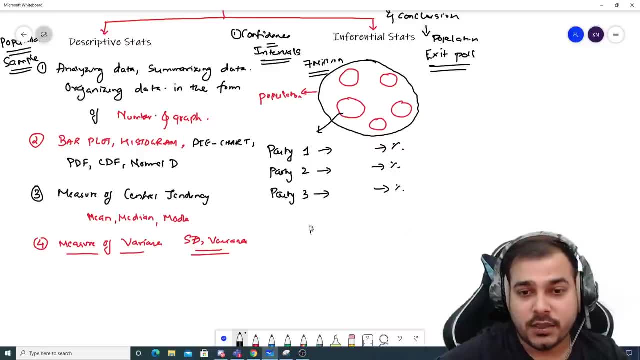 intervals. now, what are the examples with respect to some of the inferential statistics that we usually use? do let's understand that? so some of the examples that I really want to recall is something called as z-test, right t-test. we do a lot of hypothesis testing in this right hypothesis. 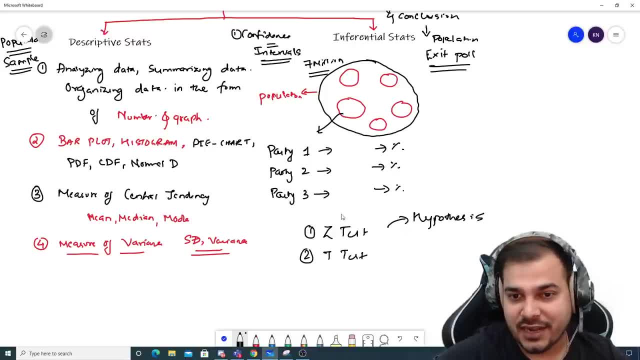 testing. right, because in hypothesis testing, in this kind of test, we also use some kind of confidence intervals. okay, someone third, one may be- chi-square test- right, we do this kind of test. these are some of the examples with respect to inferential statistics that we usually perform. 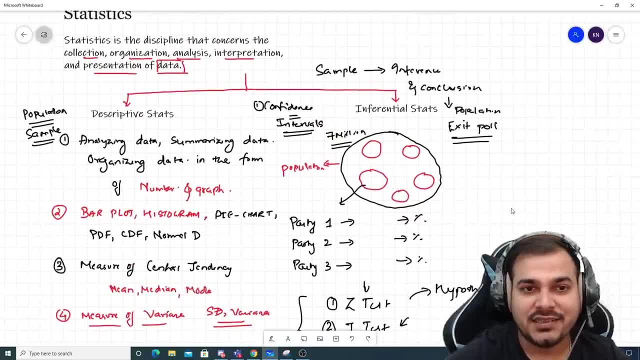 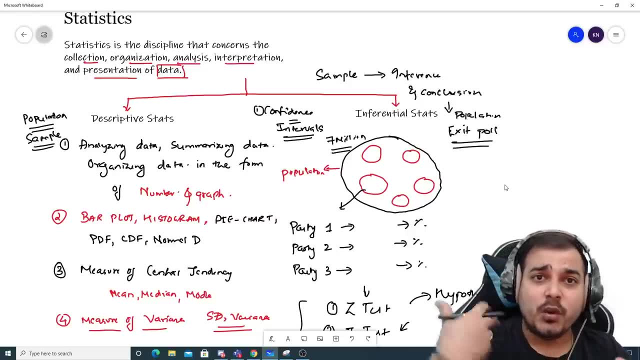 so, in short, if I really want to understand what exactly is the difference between descriptive statistics and inferential statistics, in descriptive statistics you take the population or the sample data. you analyze the data, summarize the data, you explore that particular data. you visualize that data in the form of numbers and graphs. now, some of the graphs that you. 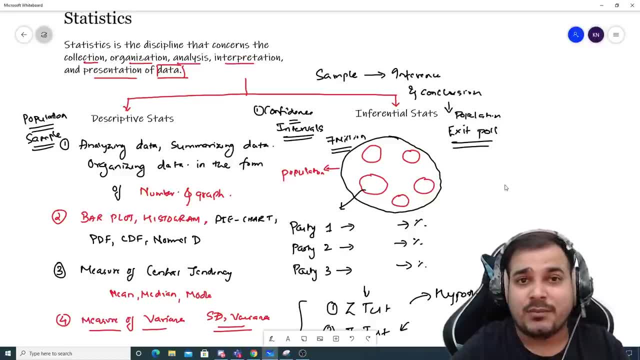 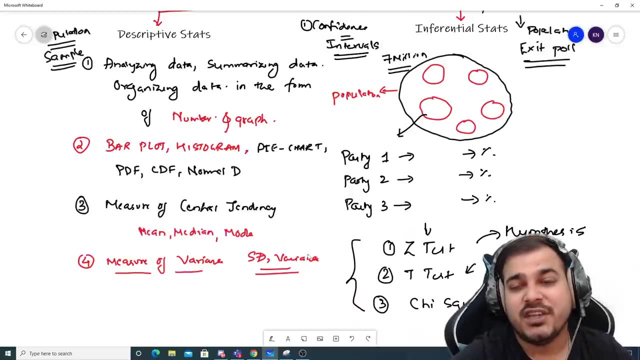 use is by the bar, plot, histogram, scattered plot, pie chart, PDF, CDF, normal distribution, Gaussian distribution, different types of distribution. you use some of the concepts like measure of central tendency, which we have discussed over here, right like mean, median mode, measure of variance, like standard deviation and variance. right then with respect to inferential. 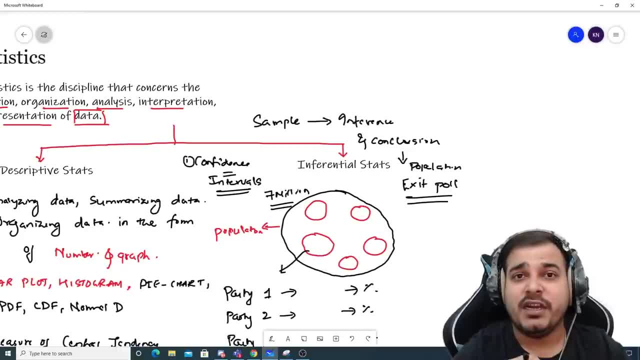 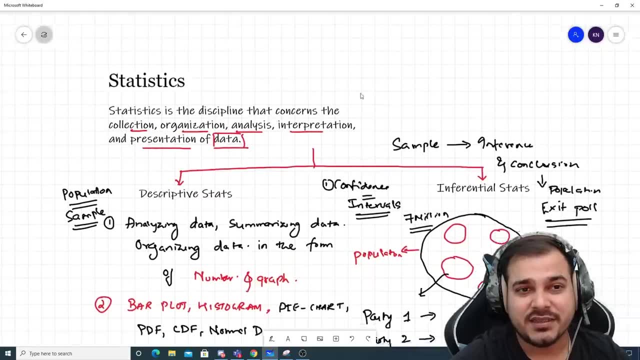 statistics. the only main aim is that we take a sample of the data, we do some kind of test and then we come to a conclusion for that specific population. right, this is only the basic difference, guys, and, as I have already defined statistics, this is how you should.